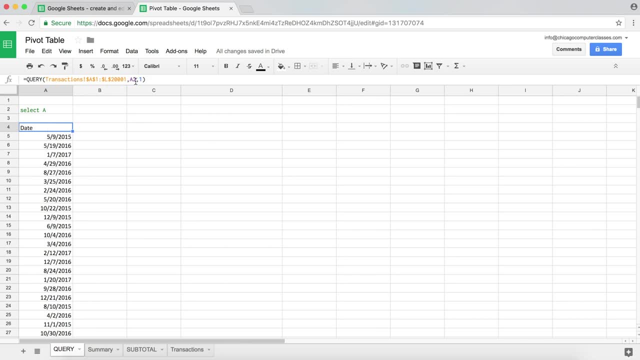 I don't have to come back and re-update this formula every single time. If you're not sure what's going on here, go back and watch the first video. So what I'm going to do: before, we used to just select the column. if I do select F, which was sales column, if you remember, this should get us that column of sales right Now. what I'm going to do: instead of selecting F, I'm going to select some F And I'll use a function. 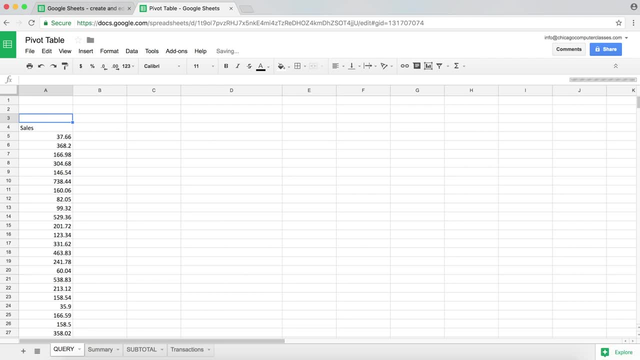 With parentheses. I'm going to hit enter Now, given it a second, you can see that we get basically the total of all sales by doing this, similar to using a sum function. What I'm going to do, I wanted to do this by brand instead of just getting the total. So after the sum, I'm going to add a space And then I'm going to use a statement called group by two separate boards And 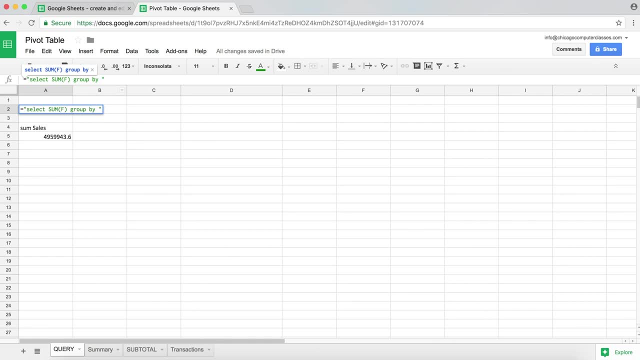 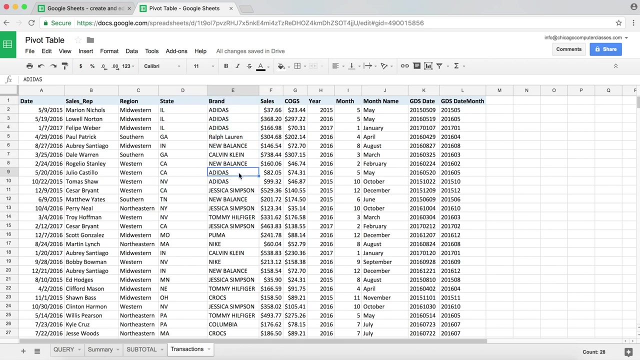 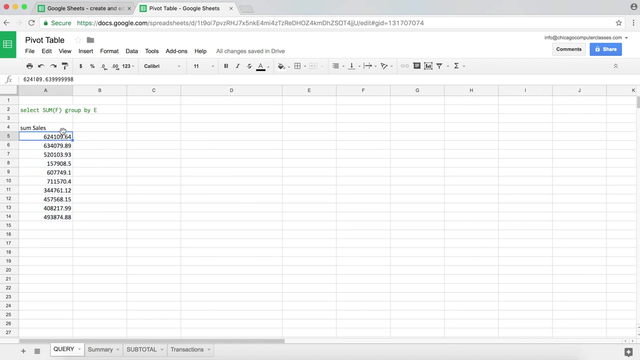 a space And we're grouping by that other column, which I believe was E if I'm not mistaken. we'll have to go back and check. So I'm going to type E, We can see. we get some numbers. So I'm going to go back here And look, E is actually the brand. So going back here, we get some totals. right, That's our totals. Now the problem here is that while I do have the totals for each brand, I don't know which. 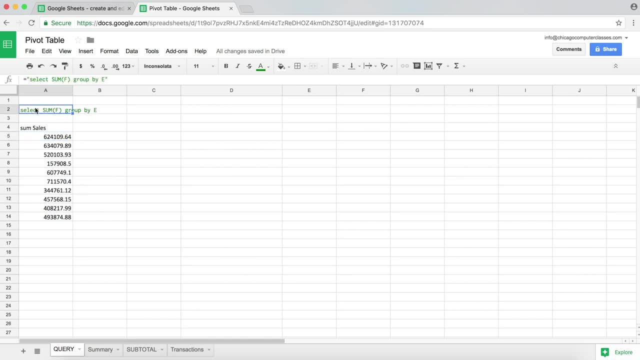 brand is which out of these numbers. therefore, when you do your select statements and you use your aggregate function- in this case some- you will have to also select what you're grouping by. so if I'm grouping by e, I want to also select that so I can see which one is which. right now you have two options. you 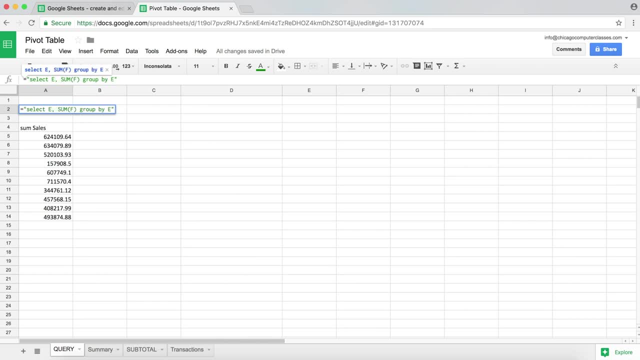 can either do your e column and comma here, or you can do the other way around: do comma here and do your e column. right now I want the brands to show up on a left, so I'm gonna do e, comma and space there. I'm gonna hit enter. give it a. 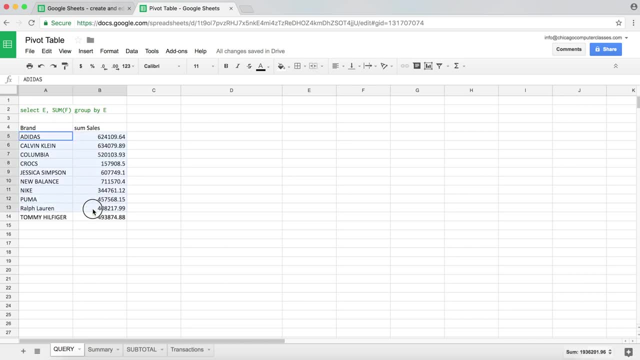 second. and there it is. that's basically our total by brand, just like that. now there are other functions we can use. instead of getting the sum, we can get the average. so if we wanted to know what's the average sale for this brand, we can simply just say a. 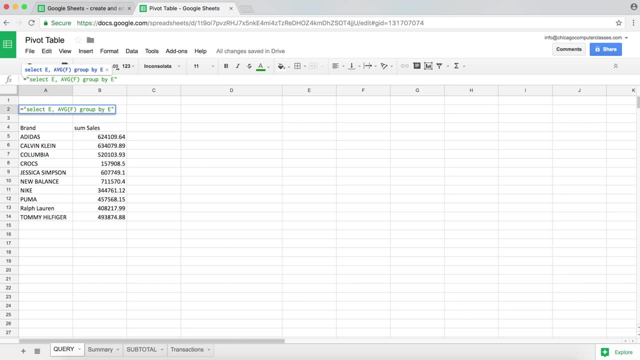 v G function and keep in mind, is not like average function in Google sheets, which is the regular average function. is a VG is our aggregate function here, so I'm gonna hit enter and that should adjust to our average sale right there. if I wanted to know how many sales we had of that brand, we can simply switch this to. 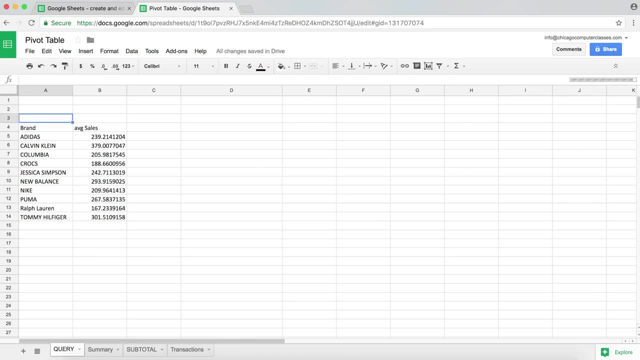 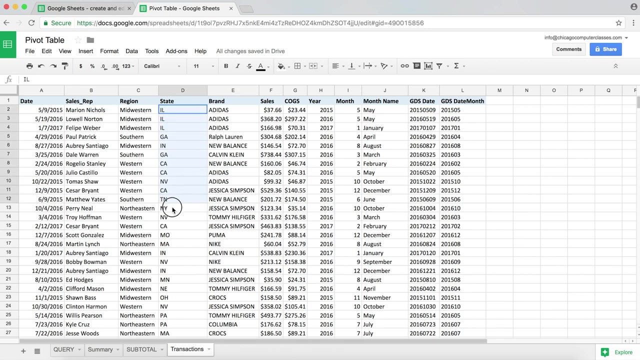 count function and that should tell us how many sales we had of each brand. there it is, that's our count function, so we're grouping by e. so if I go back, so if I wanted to basically get my sales by state, which is our D column, all I really 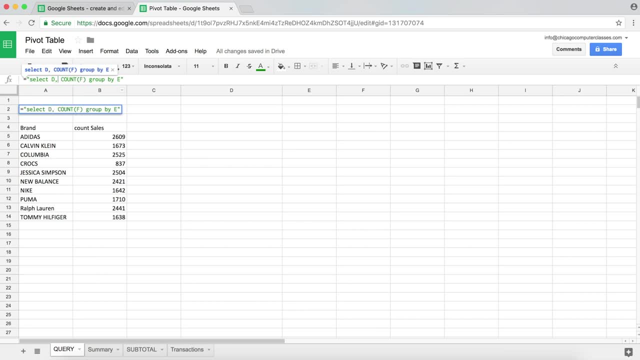 have to do is go back here and instead of e, type T, and instead of group by e, I will also group by D and instead of counting F- since we want to total will sum our F column- I'm gonna hit enter and there it is- our sales by state. this could get a little. 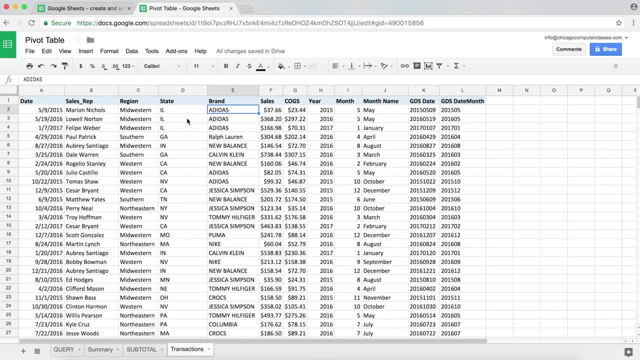 more interesting when you try to group by multiple fields. so maybe what we want to do, we have our. we want to first break it down by region and then, on a second level, we want to break it down by state. so the region is the C column. so first, 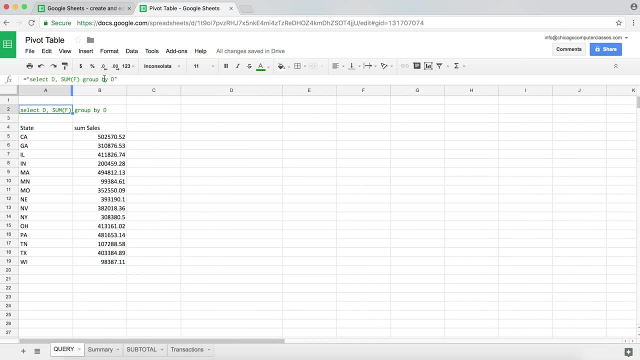 I'm gonna go back and update this and just use the C column to get a very simple and plain report, like we did before, and this should break it down by region and each region. we should have multiple states right now. I want to break it down and see in Midwestern what 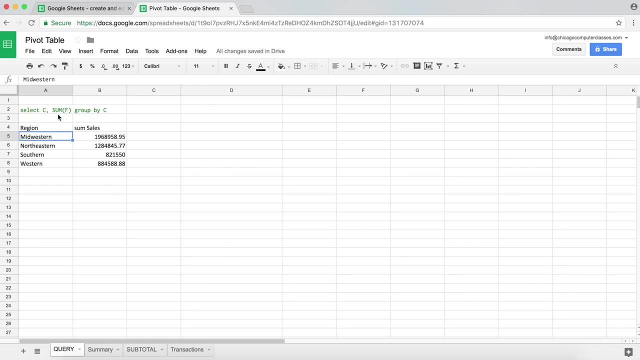 are the states that we have and how much the totals are. so the state was D column. so I'm gonna go back, I'm gonna after group by C, I'm gonna do comma and do that D column and since I want to see the results, I'm gonna have to add D. 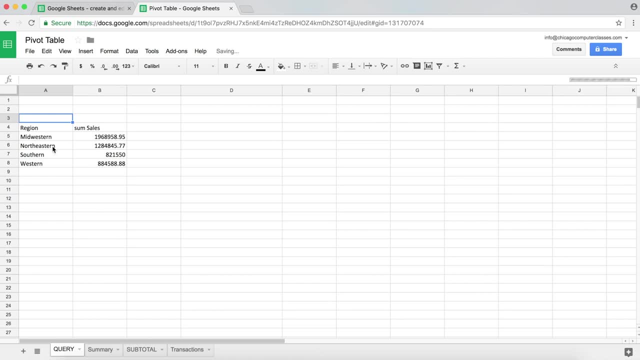 column as a select column as well. so I'm gonna hit enter, give it a sec and there it is. we have our Midwestern and you can see the states right there, and then we have the next one with our states and then next one with our totals, so we can. 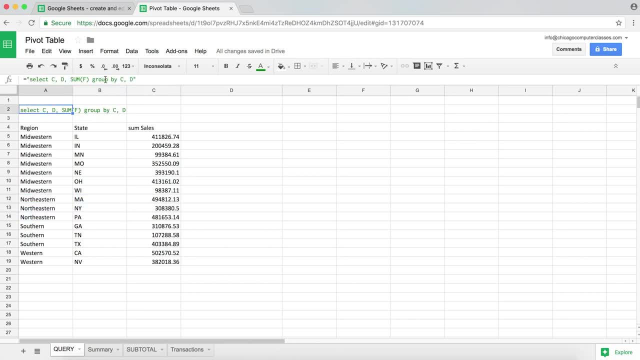 basically do both so we can group by by multiple and keep in mind that the order matters. so because I placed C as the first group by, first it does: Midwestern is the higher level and then the inner level. inside of Midwestern that's gonna be the D column. 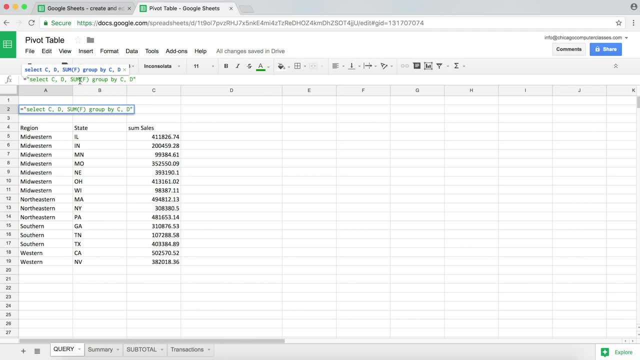 which is my states, and I'm getting my totals and obviously instead of sum you can do the average right or any other function. hopefully that makes sense. it's kind of simple. so I'm gonna go back and do comma and do comma and then I'm gonna 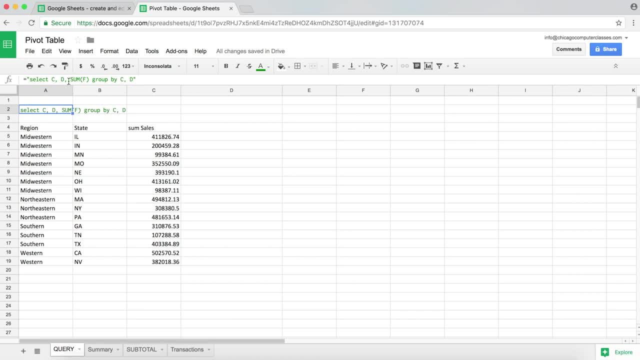 similar to how you do pivot tables, and we'll talk about like pivot functionality as well in a later video. finally, let's do one more thing. so let's say I also want to get the average. that's sale. F column hit enter and now we have both the sum and the average, and obviously I can do the count, to just do. 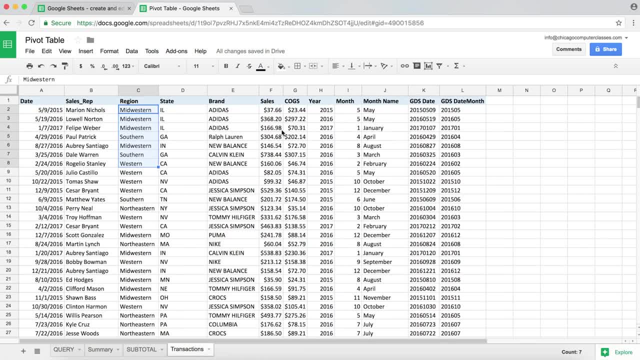 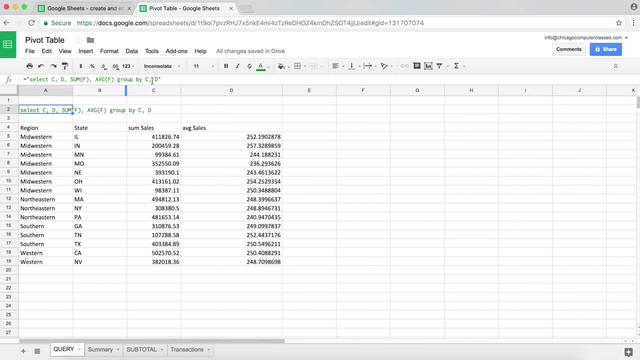 column. I'm gonna go back here and I'm gonna do the average, the sum, the average of our sales, and let's also do the sum of our cost of goods, and I'm going to do J cost of goods and I'm going to come back here. 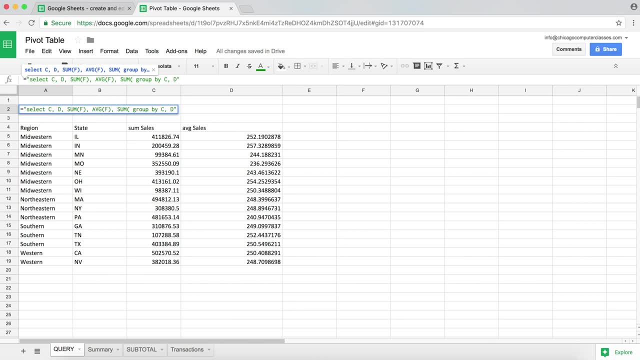 for got what the column was, so I don't know. I guess it was G. let's give it a try and I'm gonna hit enter and then I'll go back and take a look what's going on there. so yeah, that was actually right. so that's our sum of cost of goods, so we can actually summarize multiple number calls. make sure that.